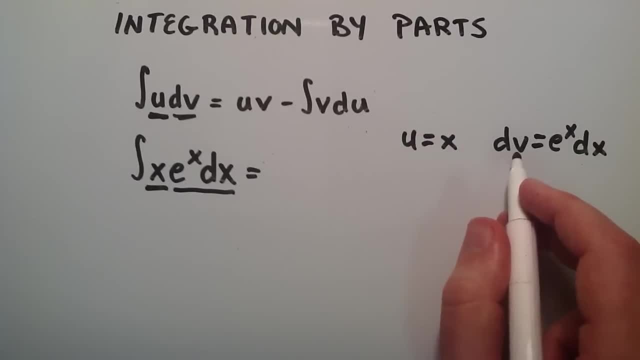 that we've got our u and our DV figured out. we also need to figure out what du is and we also need to figure out what V is. so we can figure out what du is by taking the derivative of u with respect to X, so derivative of u with respect to. 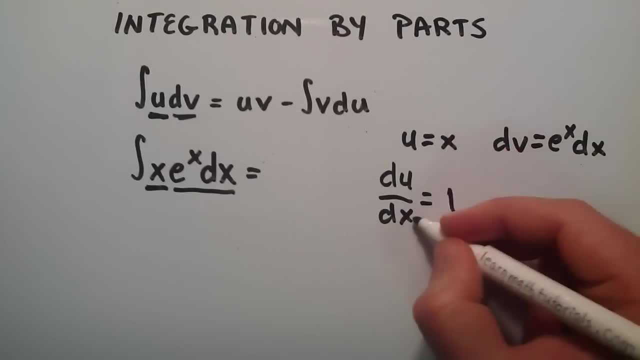 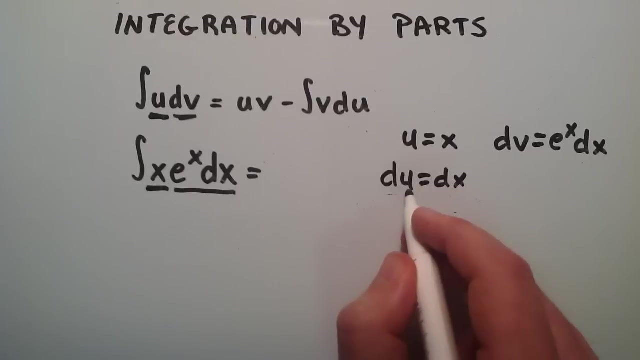 X is simply just you one, since the derivative of X with respect to X is one. and then, if we just were to multiply the left and right hand side of this by DX, this would simply become: du is equal to DX. so we've defined what du is now. so now let's go. 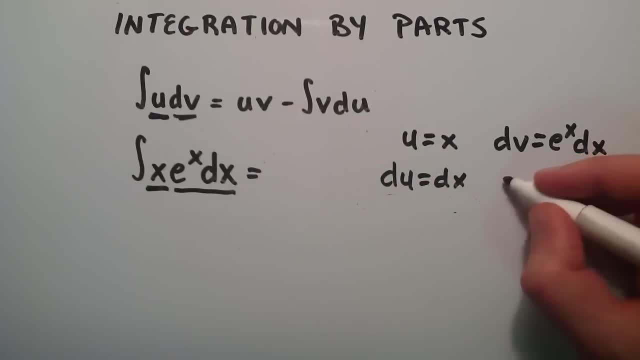 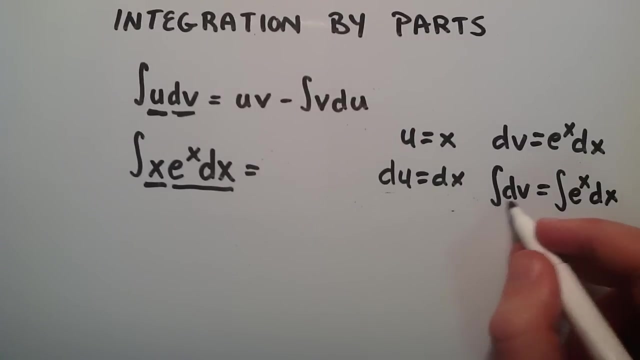 figure out what V is going to be. so if we were to just integrate the left and the right hand side of this right here we would have: the integral of DV is equal to e to the X DX, the integral of e to the X DX. and then if we integrated this side, 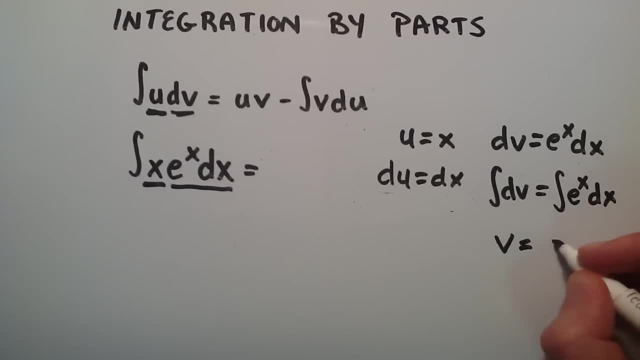 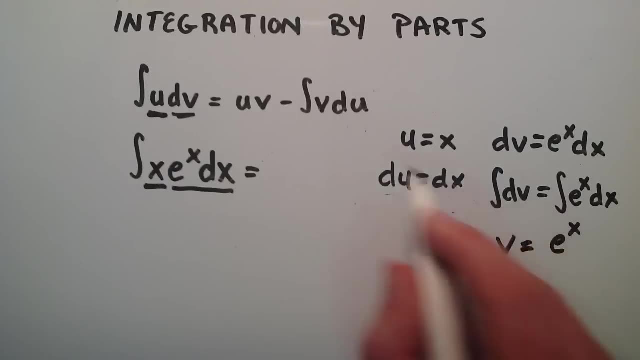 we simply have V. if we integrate this one, we have e to the X plus some constant, but we're not gonna worry about the constant right now. so this is our V. V is equal to e to the X now. so now we have all the parts we need. so 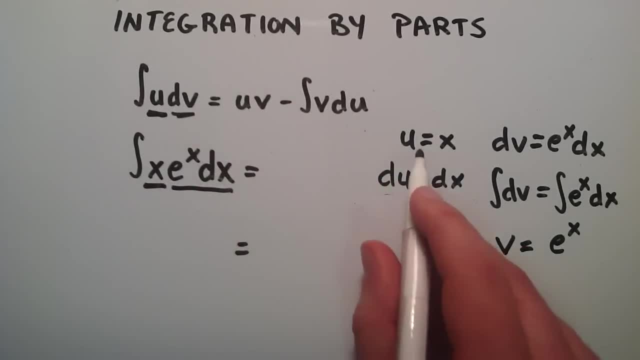 basically this is going to equal you times me with the axe. V is equal to e to the X. so this is our u times me, right here. And then we just subtract the integral of v times du. v was e to the x and du was dx. 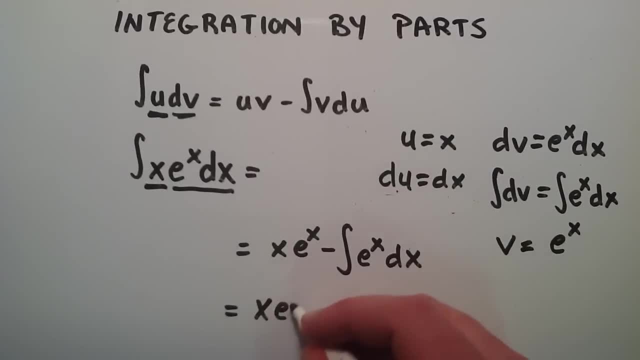 So this simply becomes x times e to the x, minus the integral of e to the x with respect to x, which is simply e to the x, And then we can go ahead and add our constant term here. So this is our answer now, and we can actually simplify this a little bit. 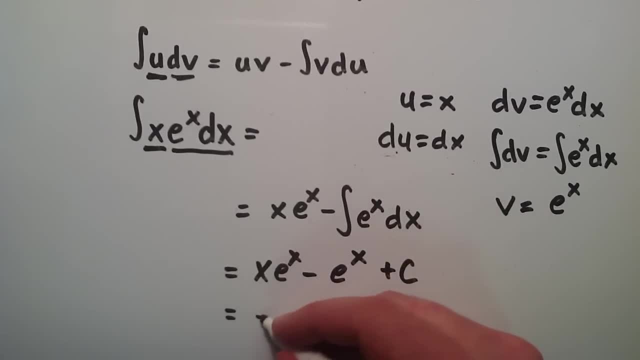 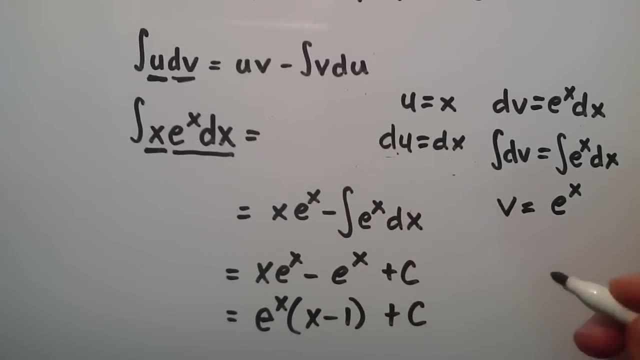 We can factor out an e to the x out of these first two terms. So this becomes e to the x times x minus 1, and then that's plus some constant. So we went ahead and just solved the integral of x: e to the x with respect to x. 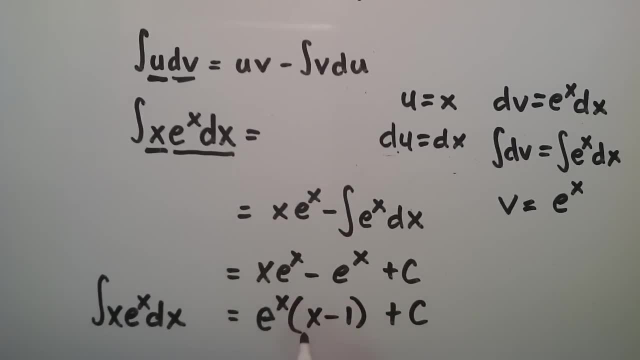 And it turns out that it's equal to e, to the x multiplied by the quantity of x minus 1 plus some constant. So this is the solution and we got that by using integration by parts. So I hope this example helped you guys understand how to use integration by parts. 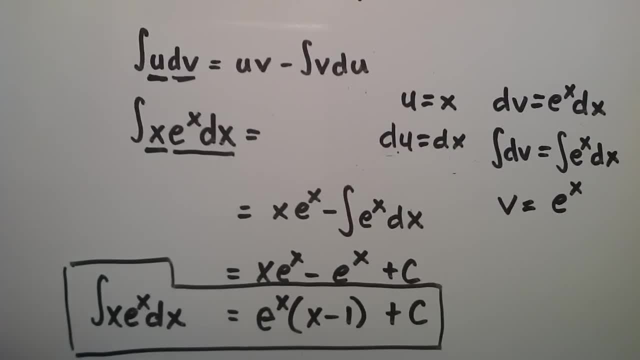 I appreciate you guys watching. I hope you have an excellent day and if you haven't already, don't forget to subscribe.